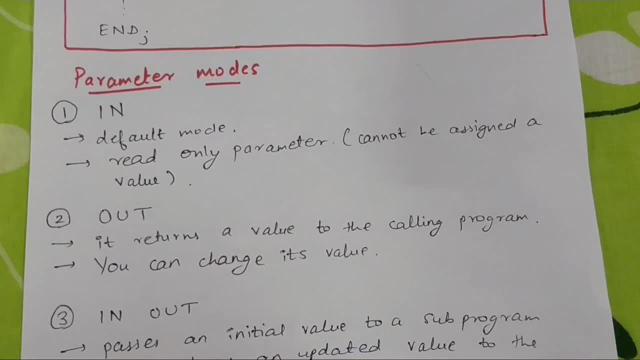 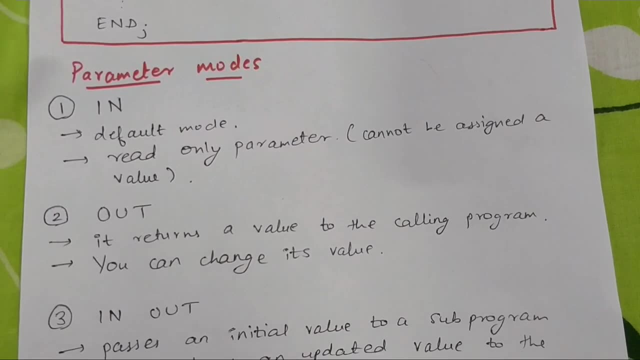 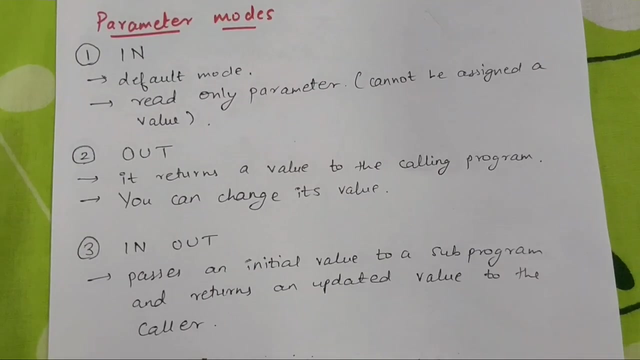 So these are read-only parameters and they cannot be assigned a value. So what this means is: in parameters they are assigned a value and the value cannot be changed. You can use the value, but you cannot change the value. You will understand these three better with an example which I will show just in a while. 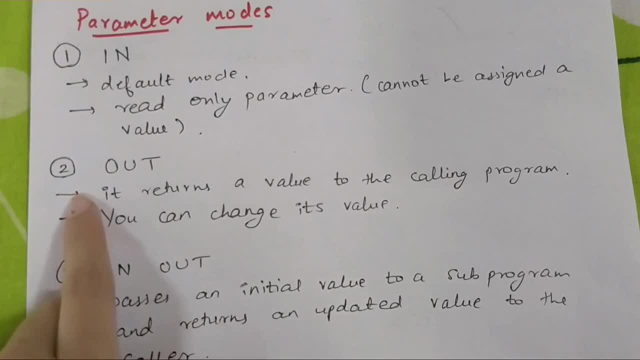 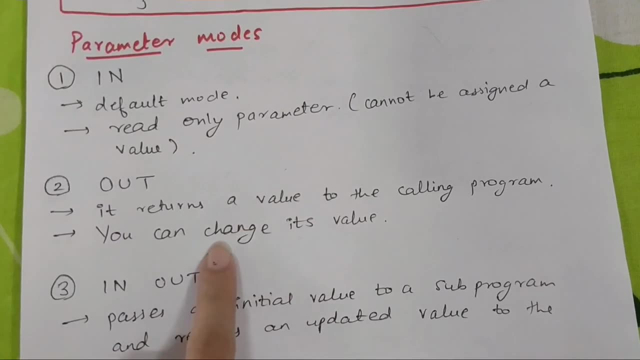 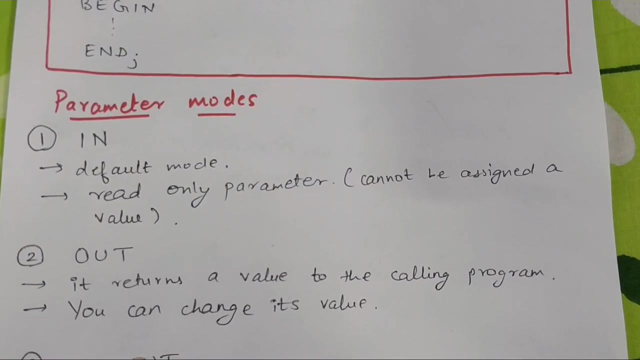 Okay Now, second is out parameter. So it returns a value to the calling program. you can change its value, So how it? so now you will get confused that, as I said, procedures, they do not return a value, They only perform an action. and here I am saying that they are returning a value. 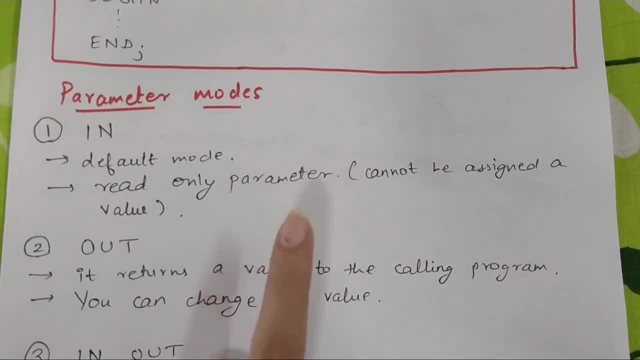 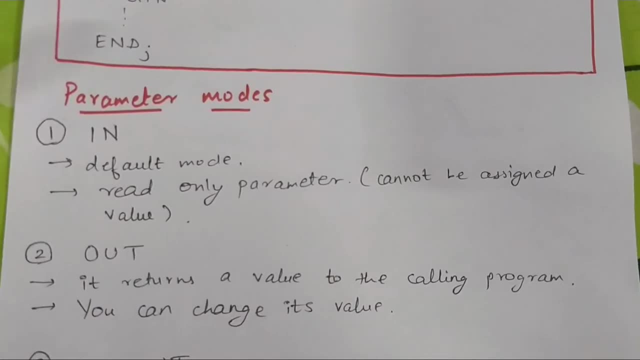 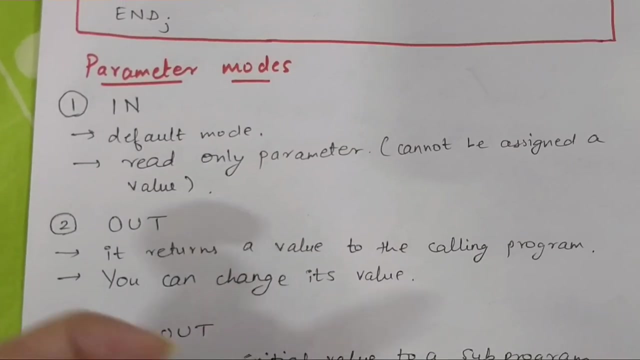 So what this means is basically: it is changing the parameter itself, changing the value of the parameter, And in that way the caller receives a value. In that way it returns a value from the procedure. You will understand this better with an example. 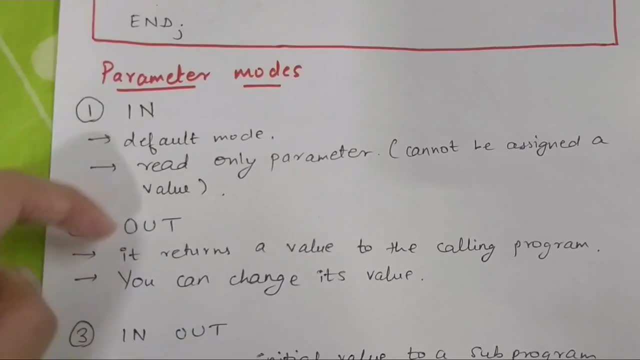 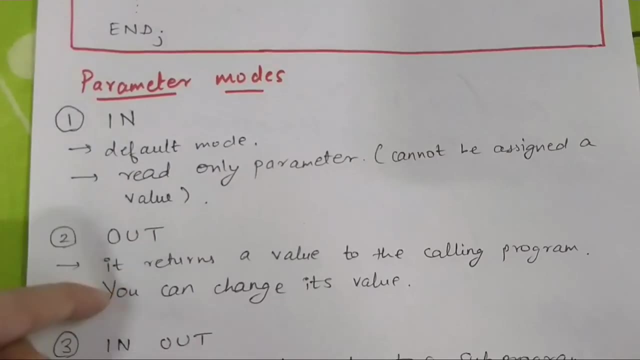 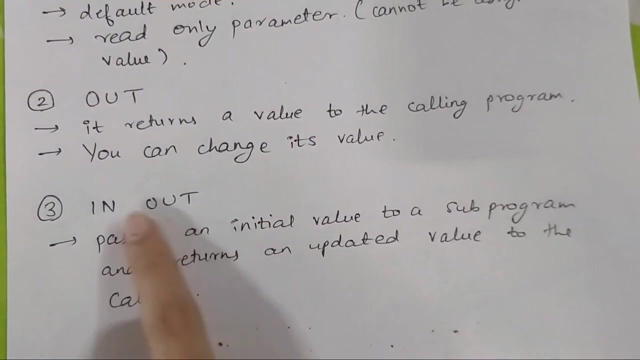 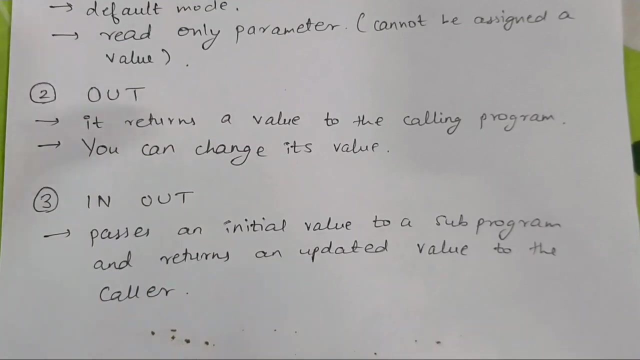 Okay. So basically the difference between in and out right now you should understand, is that in the value the parameter here cannot be changed. The value cannot be changed over here, but the value can be changed over here Now in in-out parameter mode. in-out is basically both: it passes an initial value to the sub-program and it can also change that value and hence it returns an updated value to the caller. 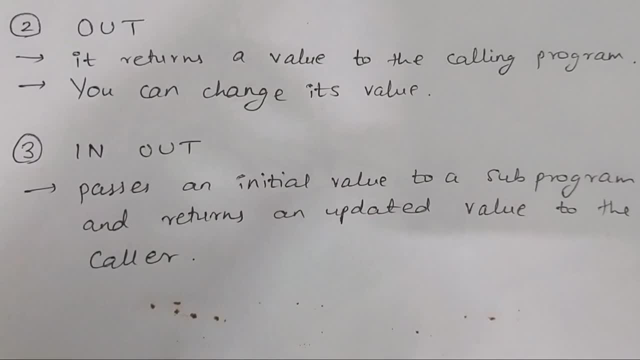 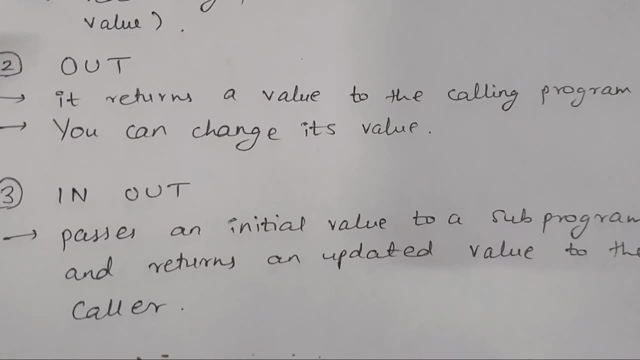 So it is only one value. Basically it It sends an initial value which you can change and in and basically return a value. Okay, Now let's see examples. Now, this is example number one. So this is the declare statement. 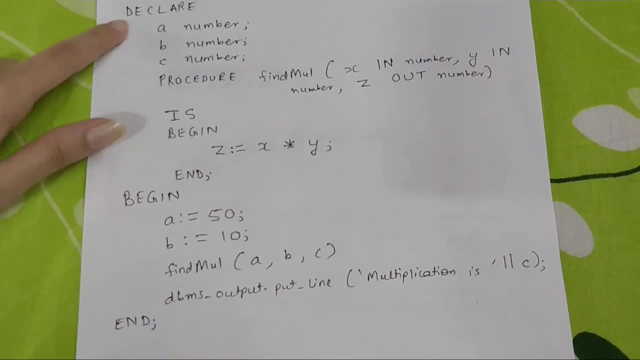 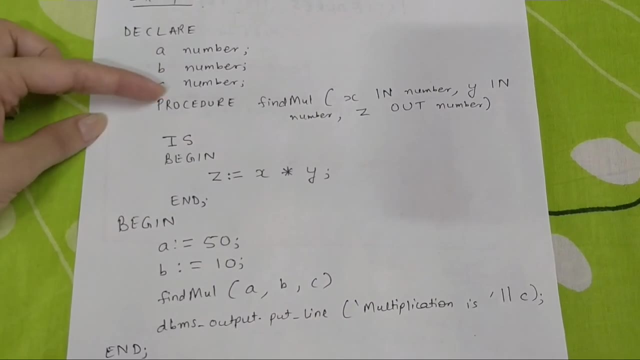 This is a normal TLSQL statement. So this is declare, This is begin, This is end. Okay, Now, in declare we can declare anything. So here what I'm declaring is ABC, three variables, ABC, which the data type is number, and then I'm also declaring a procedure over here. 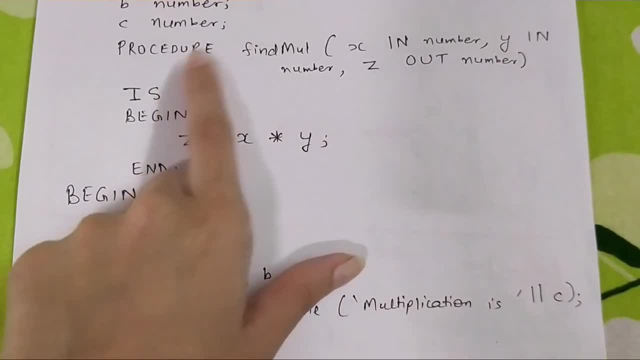 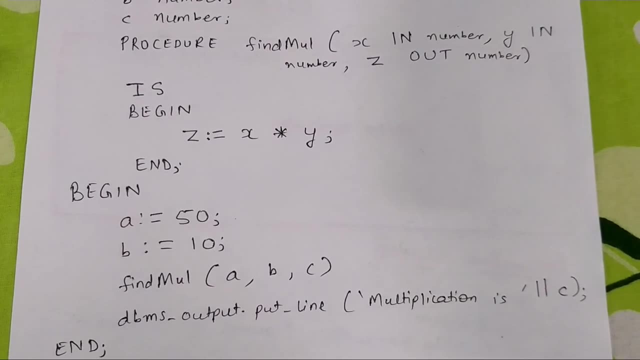 Okay, Procedure FindMul. FindMul is the name of the procedure. Basically, it's going to multiply two numbers and we'll get the multiplication. It will return a value. Basically the multiplication of the two numbers and how it will return. 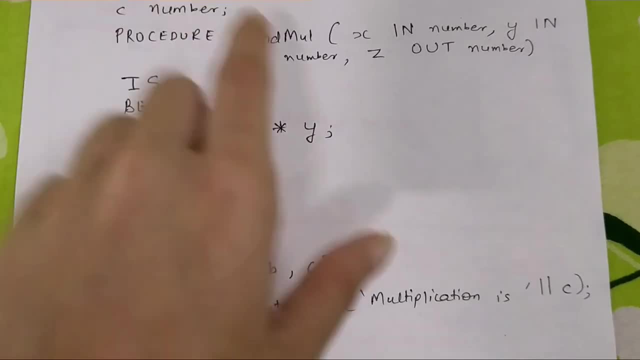 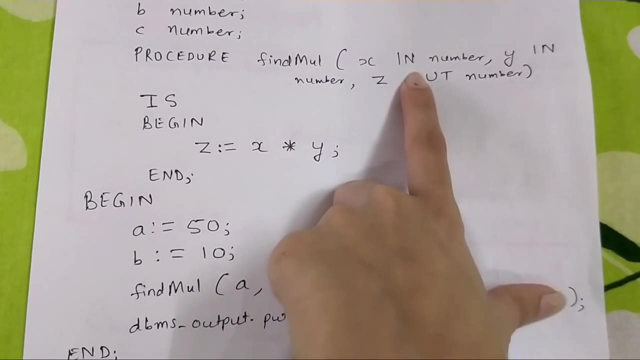 That is how we. that is what we'll see in this example. So these are the parameters between these two places. So x- x is an in-parameter number. number is the data type of x. So x is an in-parameter number. 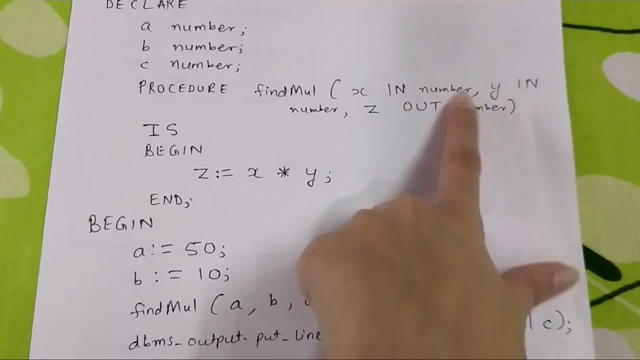 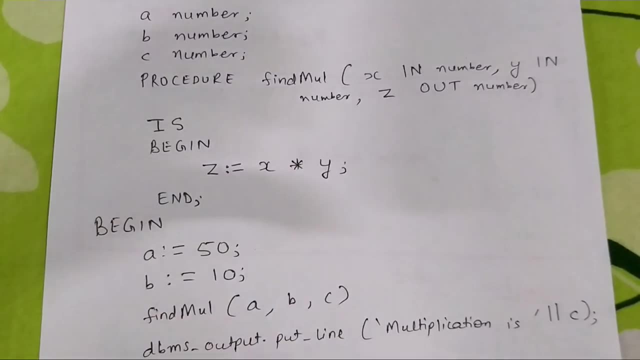 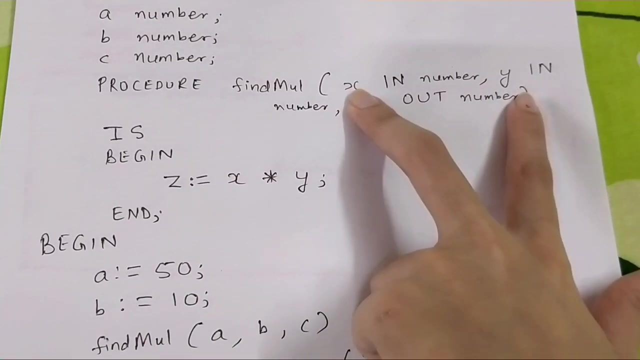 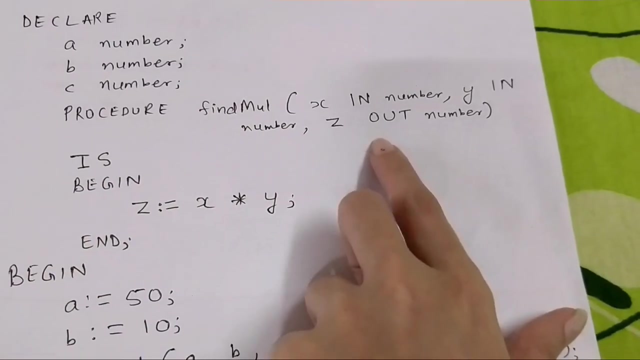 Similarly, y in-parameter, number Z, z is an out-parameter and data type is num. Okay Is begin. z is equal to x into y. So basically, basically, it will multiply x and y, the two values, and it will assign the multiplied value inside z, which is an out-parameter. 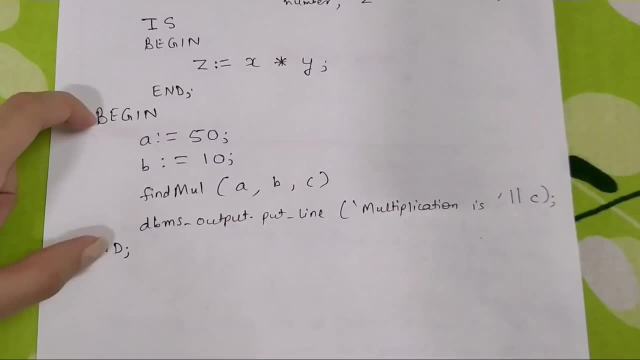 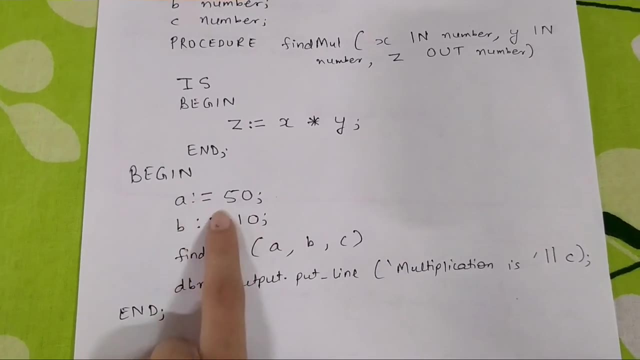 Okay, Now let's see what happens between begin and end. So a and b. a and b are assigned over here, and what are the values given to it? 50 and 10.. So a is 50 and b is 10.. 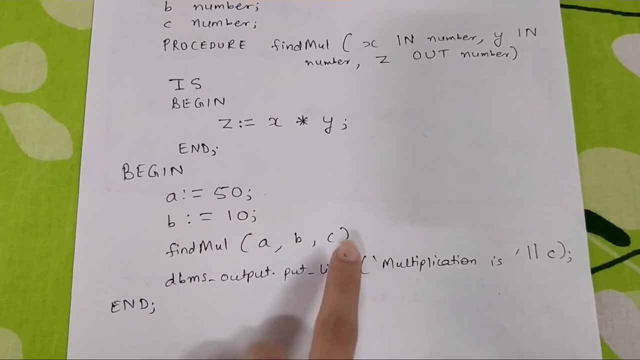 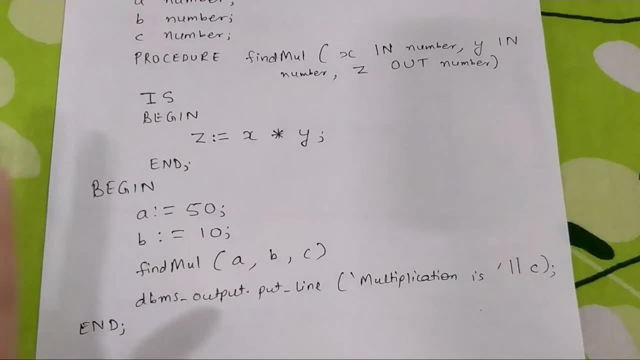 Now I'm calling the procedure: findMul: a, b, c. Okay, Now a will be given 50,, 50 will be sent, 10 will be sent and c will be sent just like that, because c is an out-parameter. 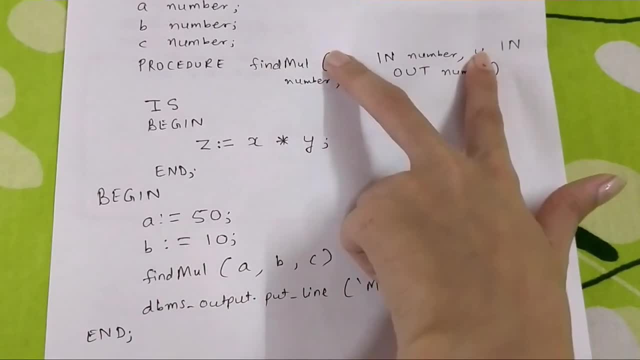 Now this same thing. this is calling here: Okay, x and y. x and y is a and b. Basically, 50 and 10 are over here. What is happening inside the procedure? 50 into 10.. 500 will be. 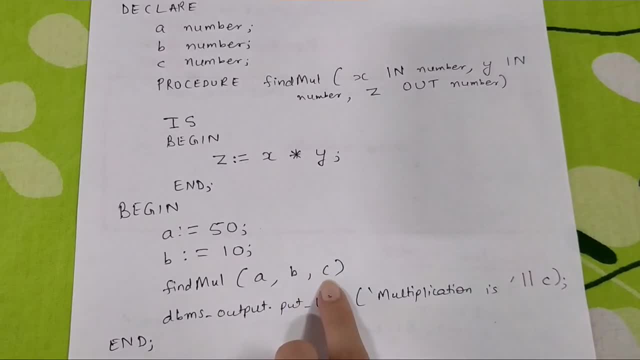 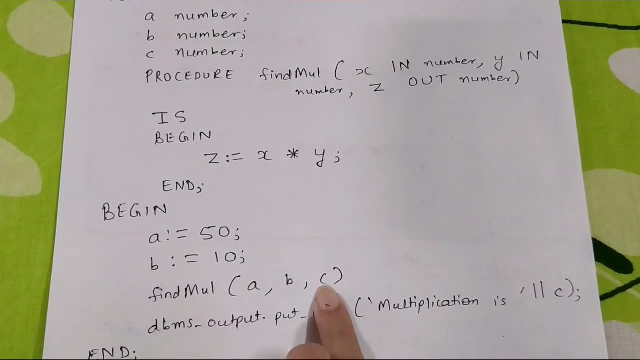 Will be assigned to z, z, z over here, which is actually c. So basically, what is z, c? So c will actually get the value 500.. Now dbms underscore output, output line. what will we print? 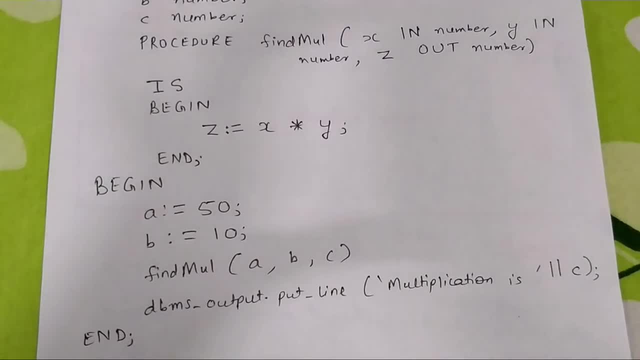 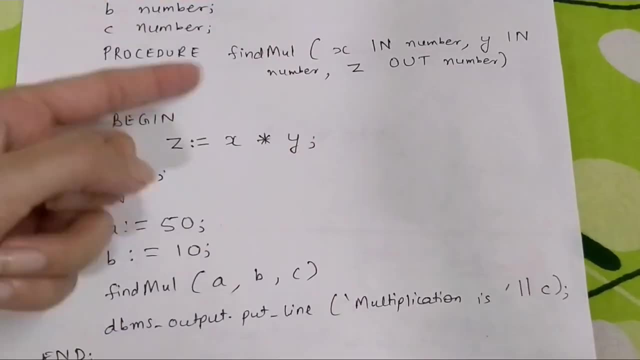 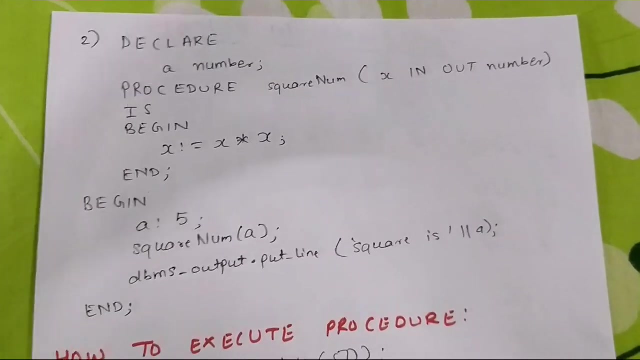 c, because c has the output. So all you need to remember is that out is used for basically getting an output from it. Okay, And in is given to give a value, give values or assign values to it. Okay. Now this is example number two. 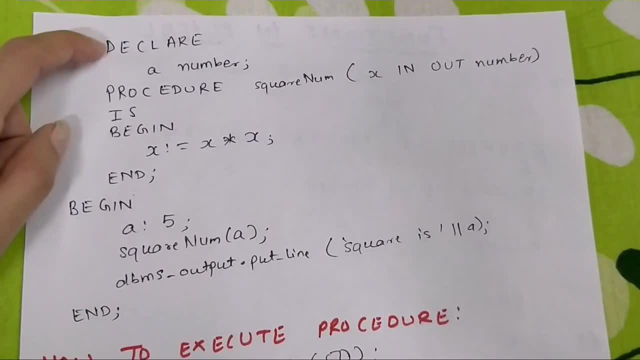 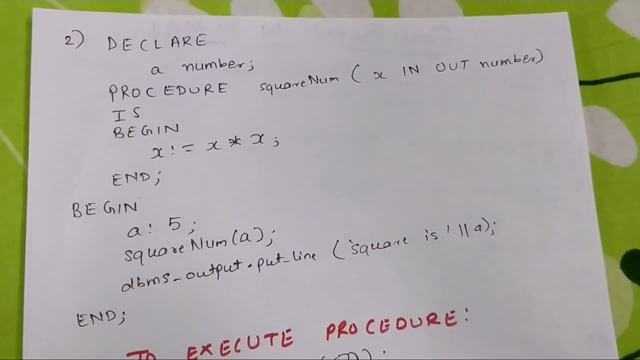 So this is declare, begin, end, Okay, So declare. What am I declaring? a is a number, Then I'm declaring a procedure. It is not important to declare a procedure over here. You can declare it separately also, but I am declaring it over here. 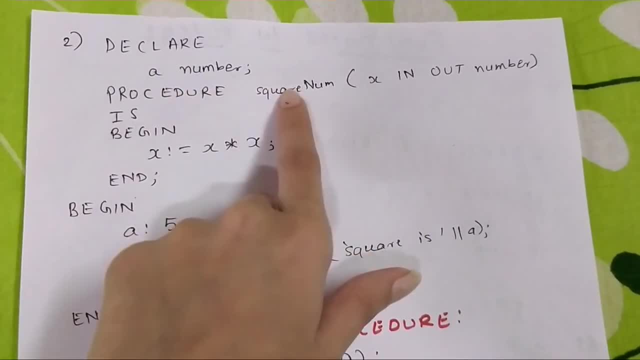 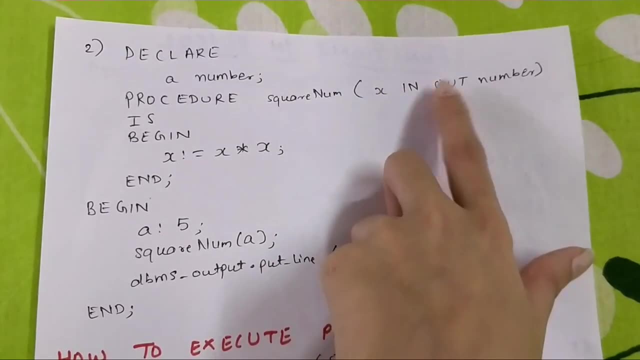 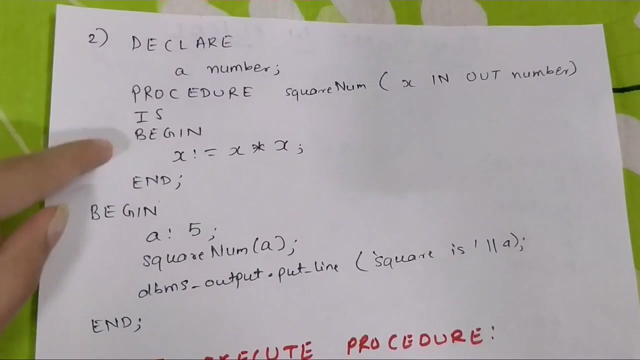 Procedure: square num. Okay, I'm declaring a procedure Square num. The name of the procedure: square num x, Which is an in-out parameter with the data type num. Okay, So here we'll see how in-out parameter mode works. 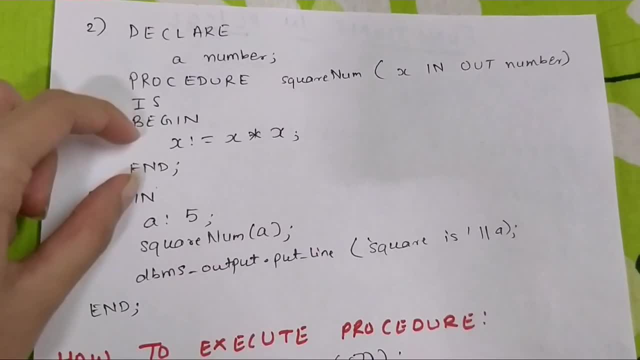 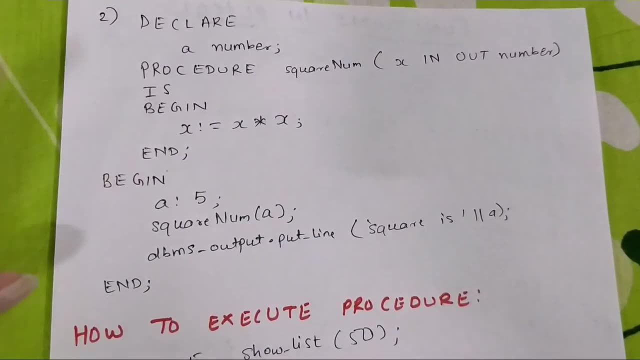 Okay, Procedure: square num. This is begin and end. Okay, What action is this procedure performing? x. x is being assigned what? x into x. Okay, Now let's see what happens between begin and end. a 5 is assigned to a. 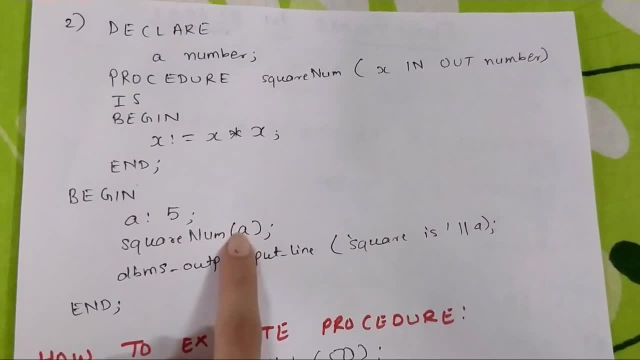 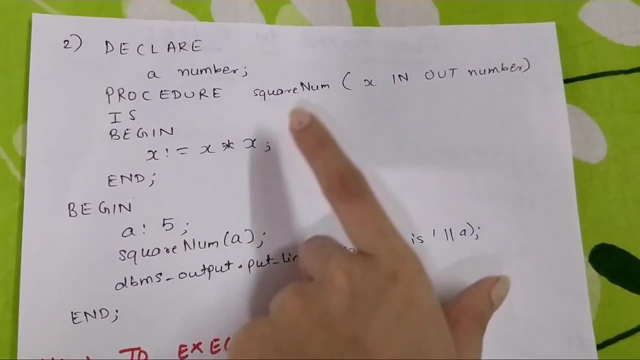 Then I'm calling the procedure square num and giving the value 5.. 5 is sent over here, Which is an in-out parameter. So in-out parameter means basically you are also sending a value. Okay, You're sending a value 5 to it. 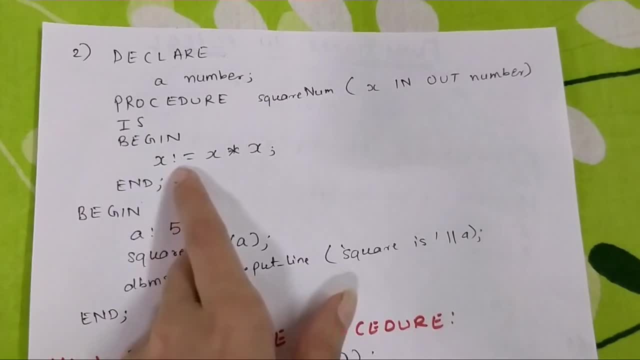 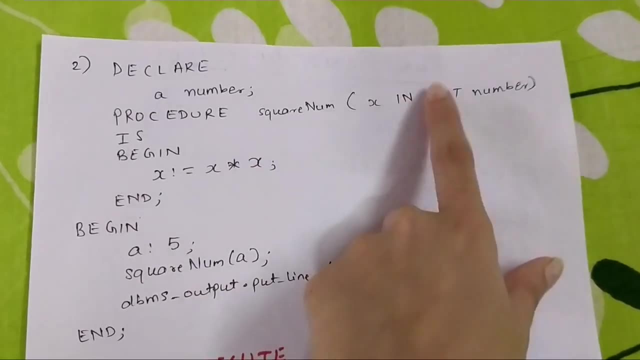 But you can also change the value, which I'm changing over here. See, I'm changing the value from 5.. But I'm changing the value of x from 5 to 5 to 5.. That is 25.. Okay, And out. 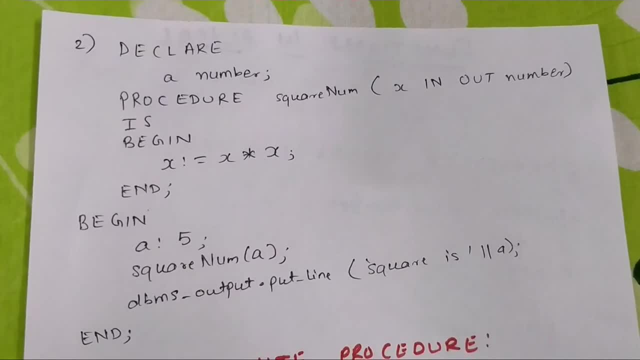 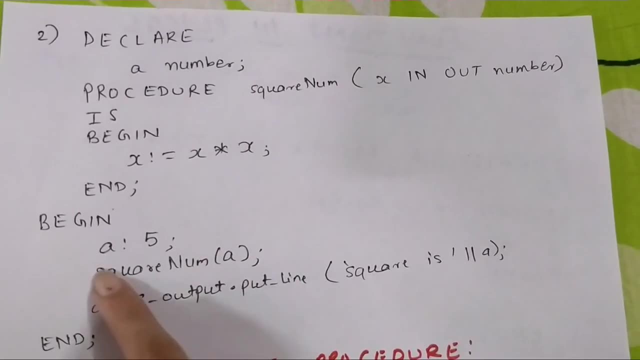 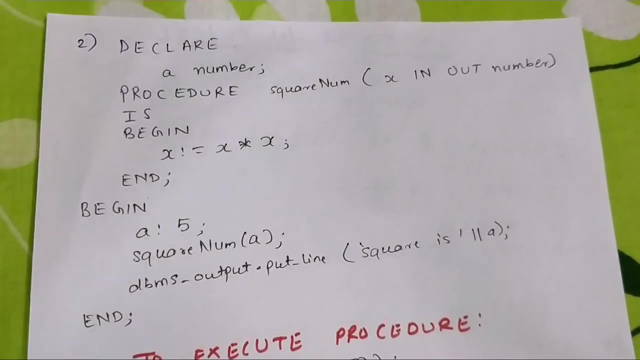 And this will be returned. Okay, This is how a value gets returned. Okay, So what will the value after performing this Procedure become? So the value of a after performing the procedure, will become 25.. From 5, it will become 25.. 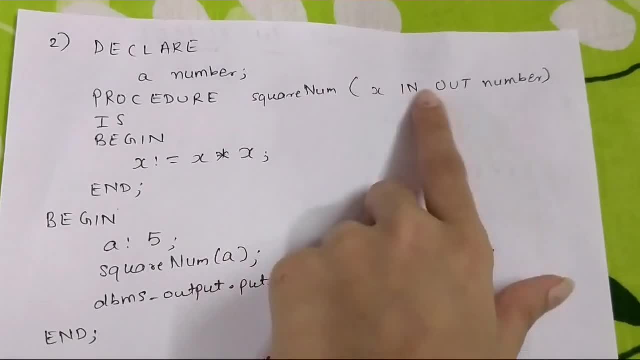 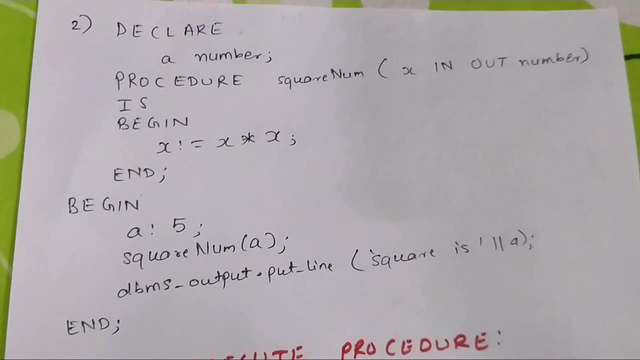 So the value is changing over here. So in-out parameter will actually assign a value, Will also assign a value, But it can also change a value and you will get an output. This is how in-out parameter works. So dbms output. and then what will I print? 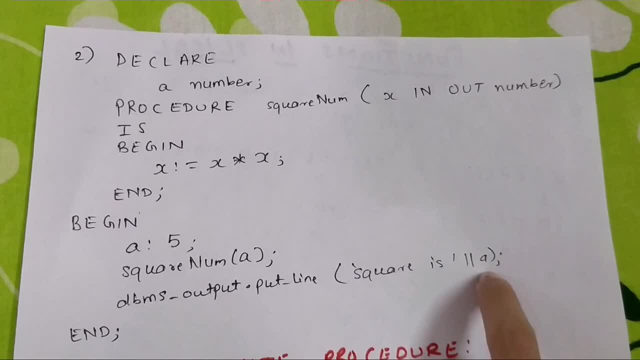 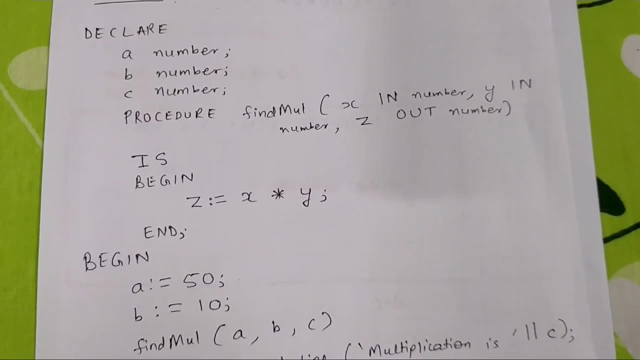 a. What will this return? 25 and not 5.. Because the value of a will change in this case. Okay, And in this case the value of a and b was not changing. Because a and b are in parameters, They cannot be changed. 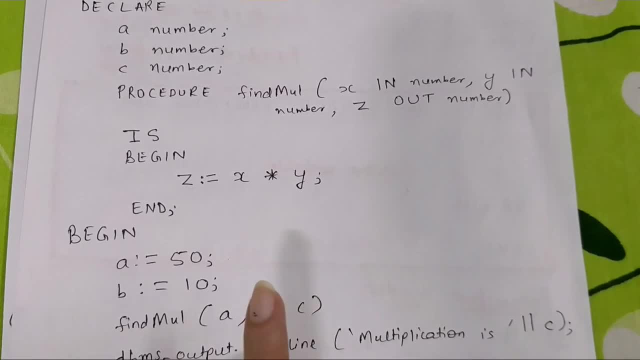 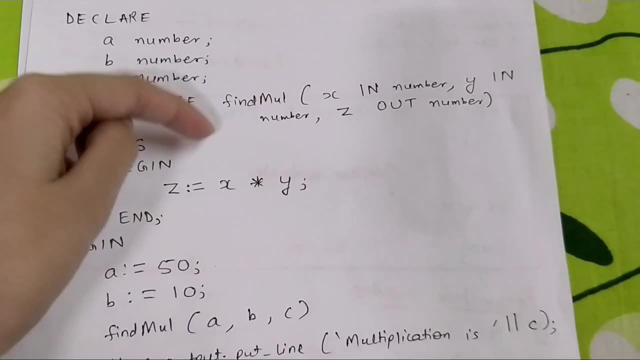 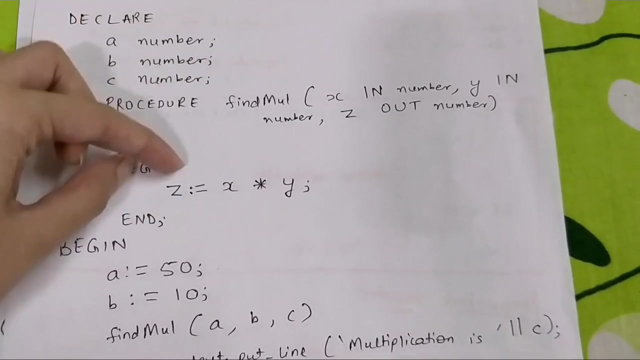 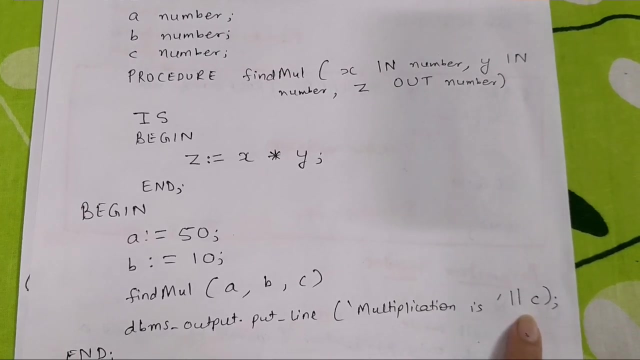 And the c was just sent over here. You cannot assign a value to c From here. from the procedure, you An answer will be put in z, Okay, Which will be sent to c, and then you can print the output. Okay. 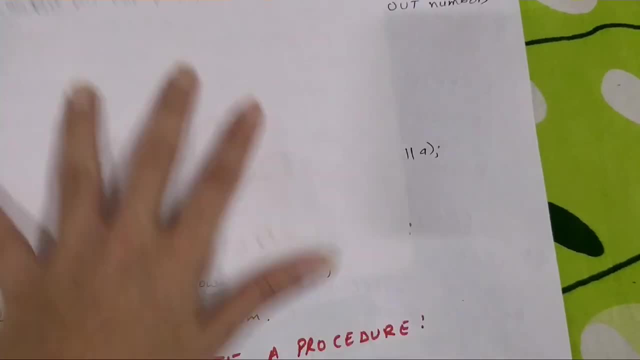 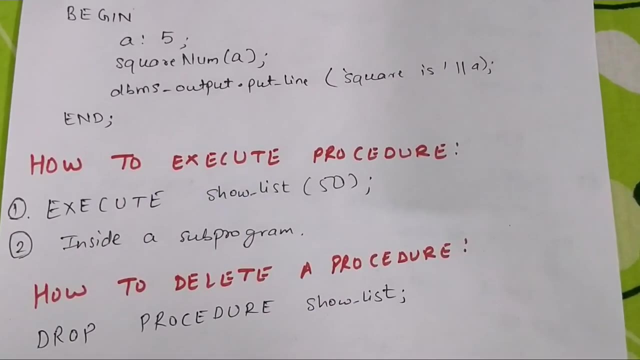 So this is what in-in parameter is and out parameter is, And this is what in-out parameter mode is. Now how to execute a procedure. So one way of executing procedure is execute whatever the name of the procedure is. So show underscore less. fifth,